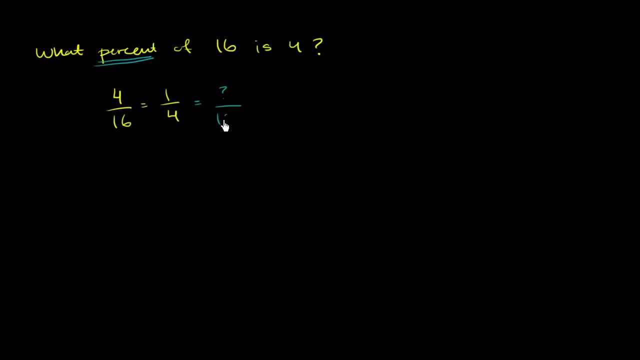 So you could say: well, this is going to be equal to question mark over 100, the part of 100. And there's a bunch of ways that you could think about this. You could say: well, look, if in the denominator 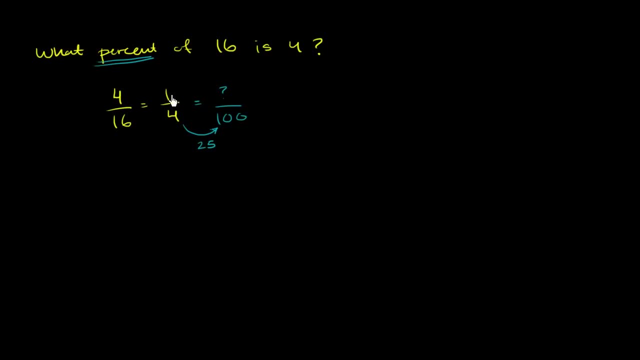 to go from 4 to 100, I have to multiply by 25.. In the numerator To go from, I need to also multiply by 25 in order to have an equivalent fraction. So I'm also going to multiply by 25.. 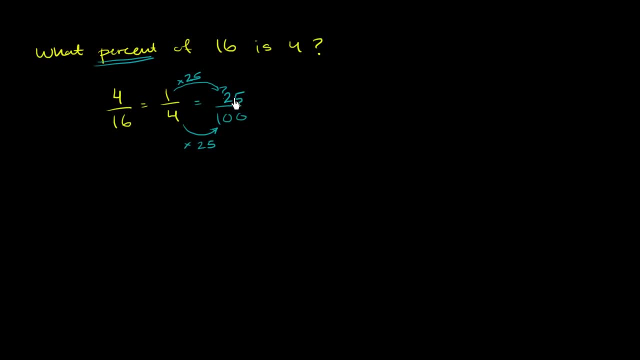 So 1- fourth is the same thing as 25 over 100. And another way of saying 25 over 100 is this is 25 per 100, or 25 per cent. So this is equal to 25 per cent. Now there's a couple of other ways. 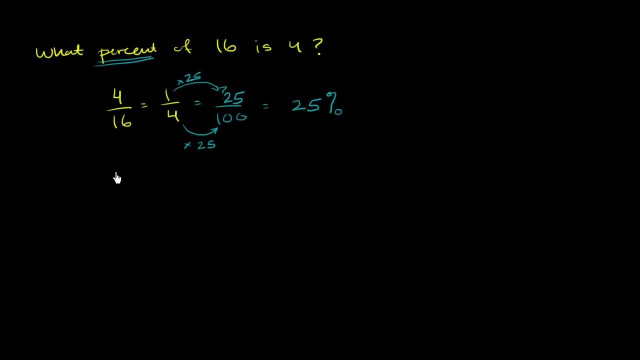 you could have thought about it. You could have said: well, 4 over 16.. This is literally 4 divided by 16.. Well, let me just do the division and convert to a decimal, which is very easy to convert to a percentage. 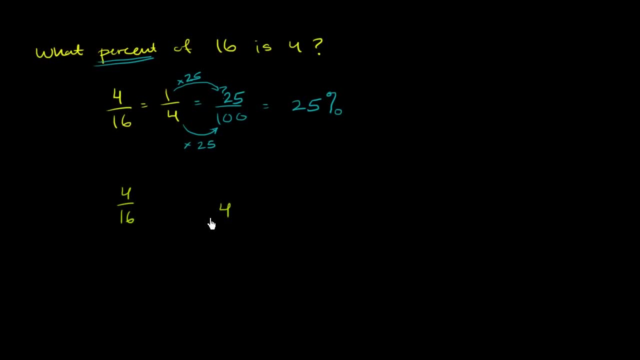 So let's try to actually do this division right over here. So we're going to literally divide 4 by 16.. Now 16 goes into 4. 0 times. 0 times 16 is 0.. You subtract and you get a 4.. 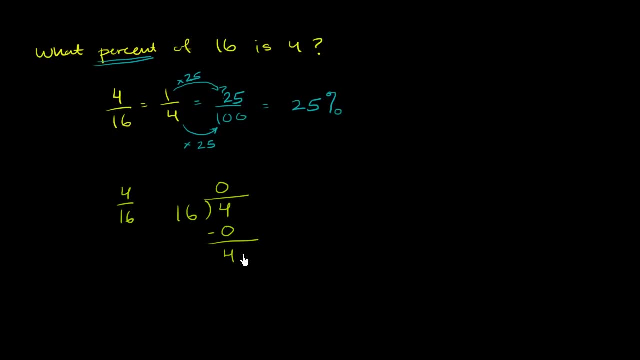 And we're not satisfied just having this remainder. We want to keep adding 0's to figure out what, to get a decimal answer right over here. So let's put a decimal right over here. We're going into the tenths place And let's throw some 0's right over here. 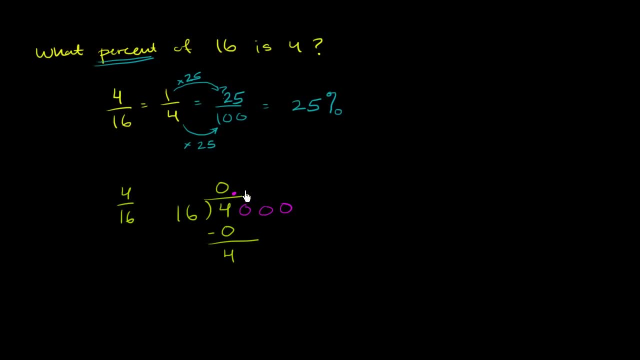 The decimal. make sure we keep track of the fact that we are now in the tenths and then the hundredths and then the thousandths place, if we have to go that far. But let's bring another 0 down. 16 goes into 40, goes into 40 two times. 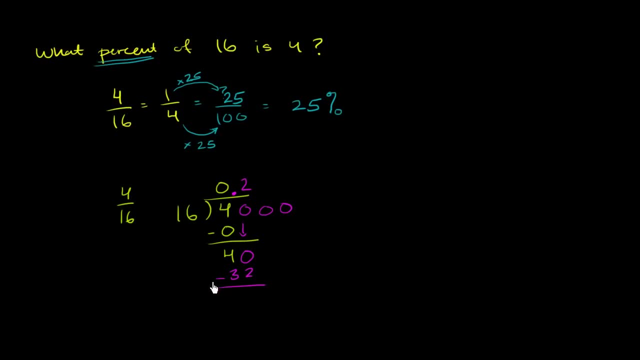 2 times 16 is 32.. You subtract, you get 8. And you could bring down another 0. And we have 16 goes into 80.. Let's see: 16 goes into 80 five times. 5 times 16 is 80.. 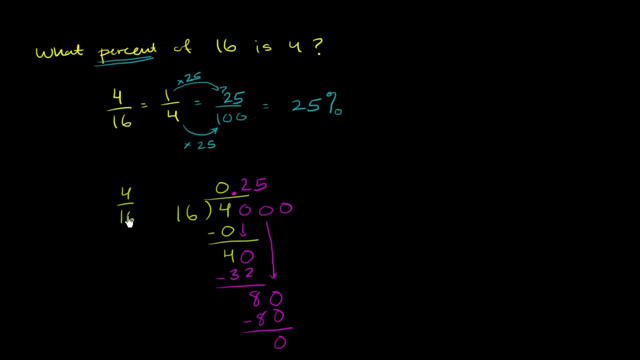 You subtract, You have no remainder and you're done. 4 sixteenths is the same thing as 0.25.. Now, 0.25 is the same thing as 25 hundredths. Or this is the same thing as 25 over 100,.